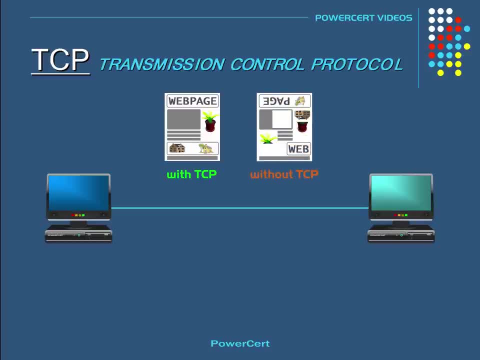 web page. without TCP, your web page could be all messed up, The images could be missing or the text could be backwards and out of order. Or if you download a file, then you might not get the entire file or you could get the file out of. 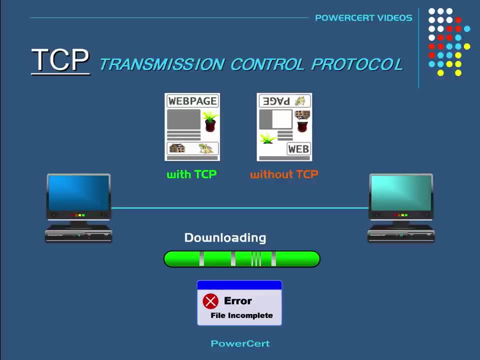 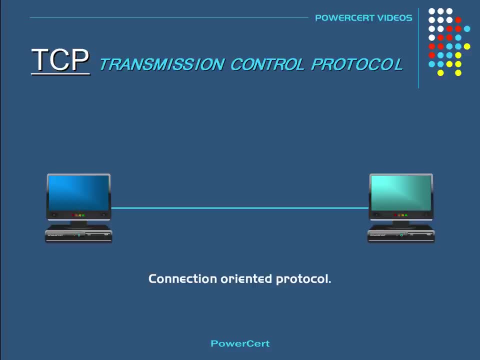 order, which would render the file useless. So again, this is where TCP comes in. Now. TCP is a connection oriented protocol, which basically means that it must first acknowledge a session between the two computers that are communicating, So the two computers verify a connection before any. 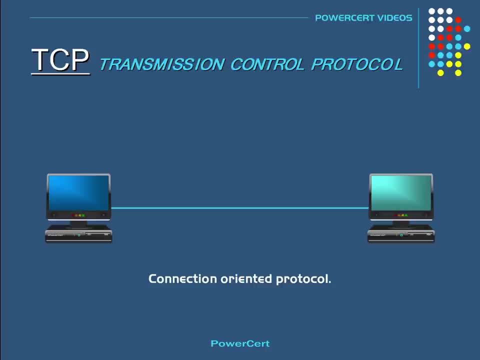 communication takes place, And it does this by using a three-way handshake. So the first step is that a computer will send a message called a ssin syn. Then the receiving computer will send back an acknowledgement message telling the sender that it has received the message. 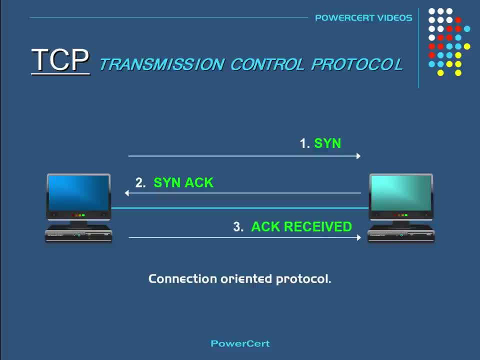 And then, finally, the sender computer sends another acknowledgement message back to the receiver And then, once this has taken place, data can be delivered. Another important thing to remember about TCP is that it guarantees the delivery of the data, So if a data packet goes astray, 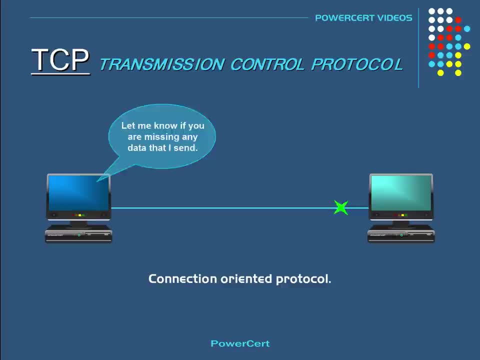 and doesn't arrive, then TCP will resend it. Now UDP is very similar to TCP. UDP is also for sending and receiving data, but the main difference is that UDP is connectionless, Which means that it does not establish a session and it does not guarantee data delivery. So when a 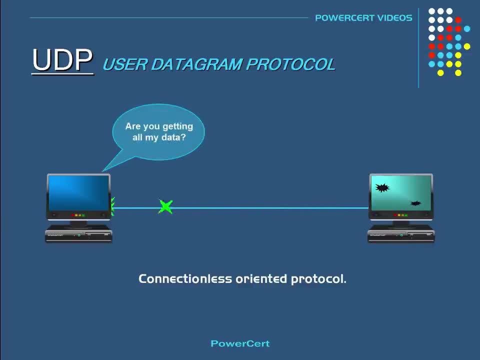 computer sends their data, it doesn't really care if the data is received at the other end. And that's why UDP is known as the fire and forget protocol, because it sends data and it doesn't really care what happens to it, as this demonstration will show. Another point to remember is because of